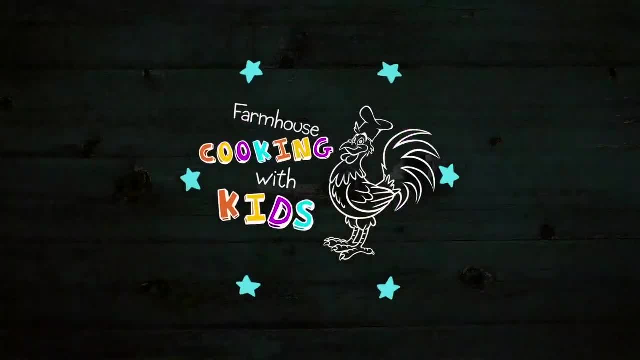 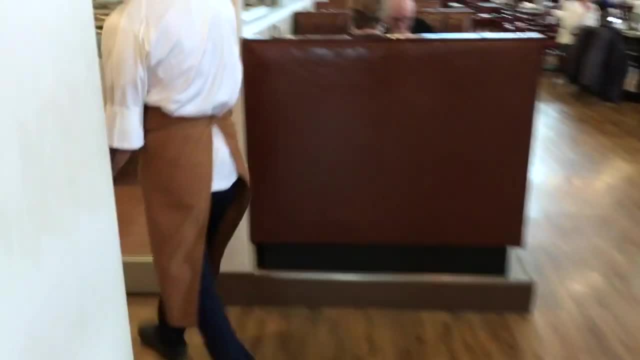 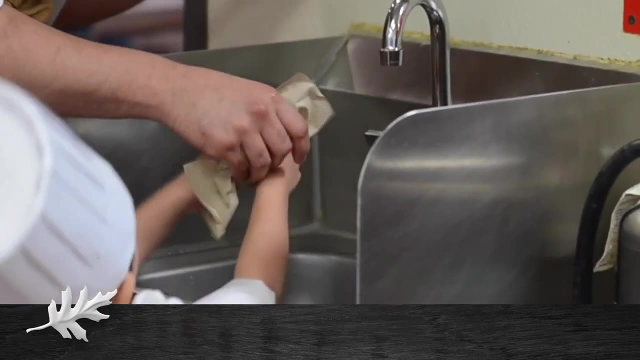 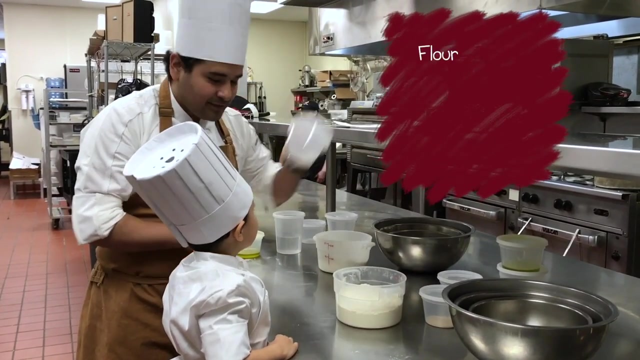 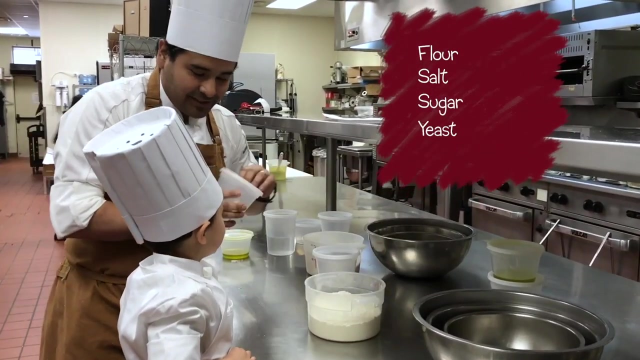 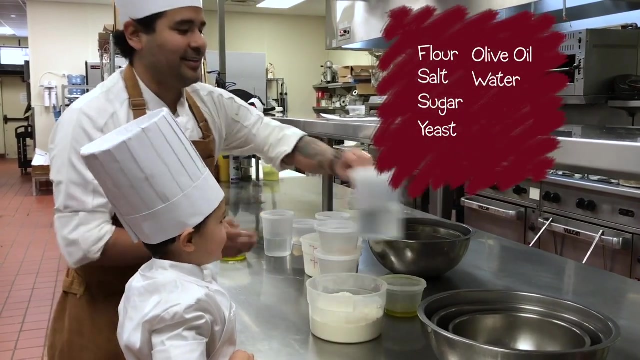 Music. What we have here is eh, eh flower. eh, we got eh flowers. What did we pick? Is it salt? Yeah, What is this? Sugar? some yeast, olive oil and what is this Water? There we go. 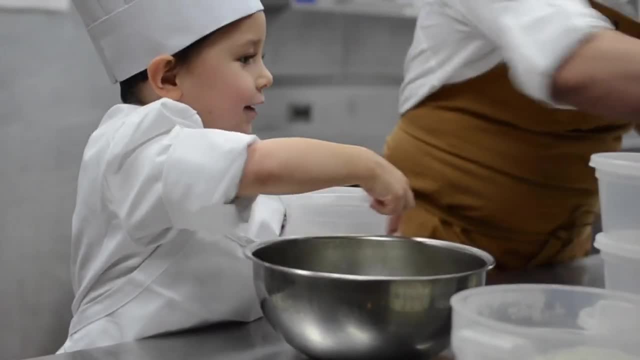 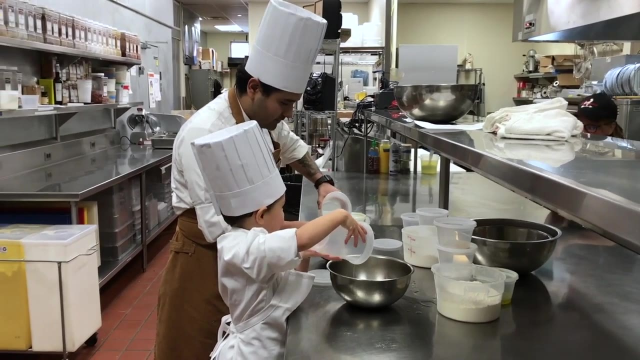 So I think it's important to cook with your kids because you're going to spend quality time with them, and then show them the importance of being organized, Like the French they always said: you know mise en place, you know keep everything organized. 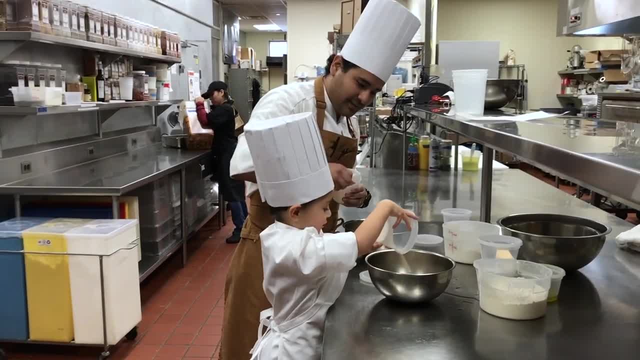 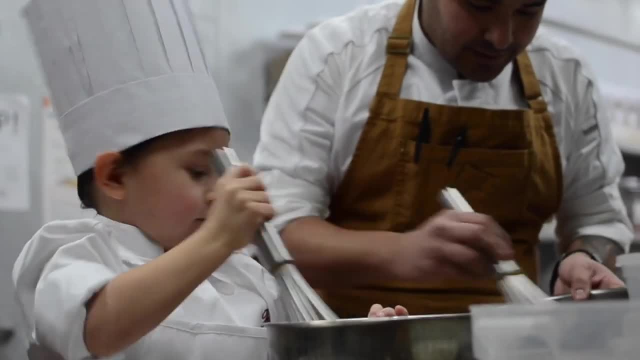 In the kitchen. it's to be organized. It's about organization. They're learning new skills. They're learning different kind of food. They might sometimes don't eat it, you know. and then you're showing them the way it's made. 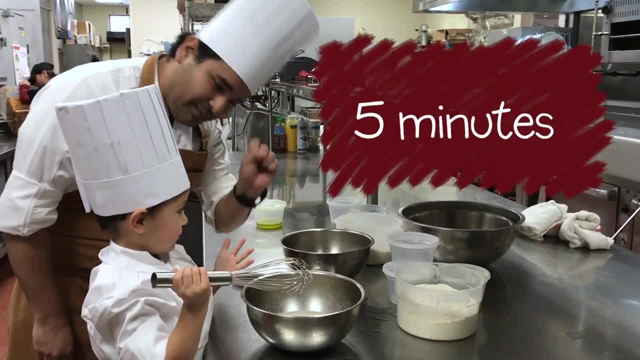 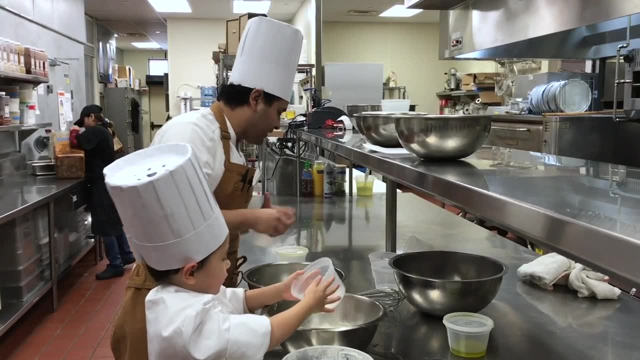 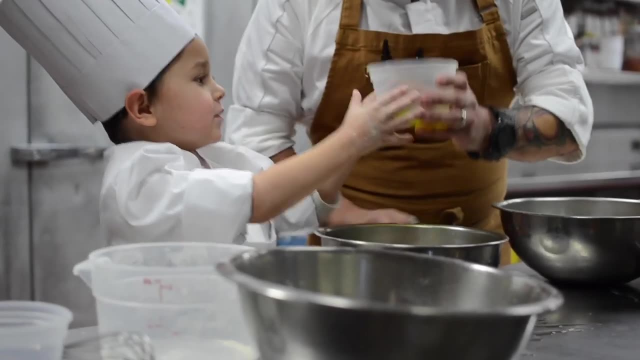 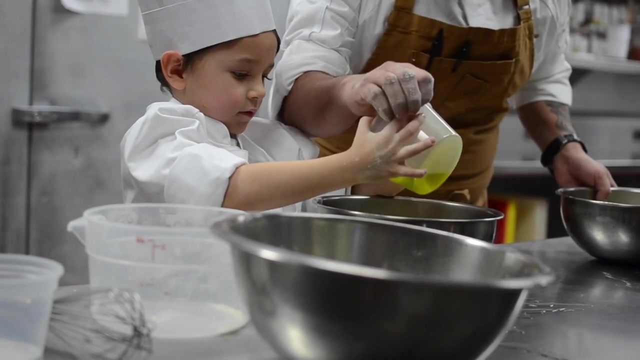 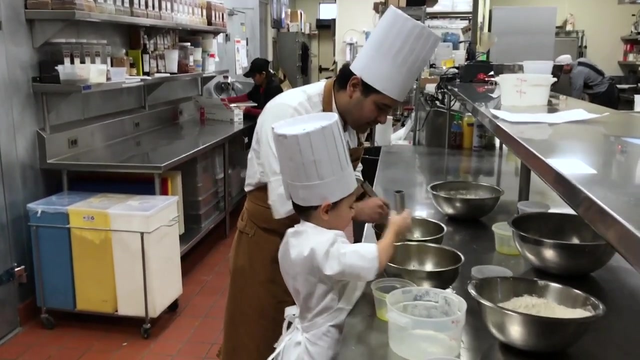 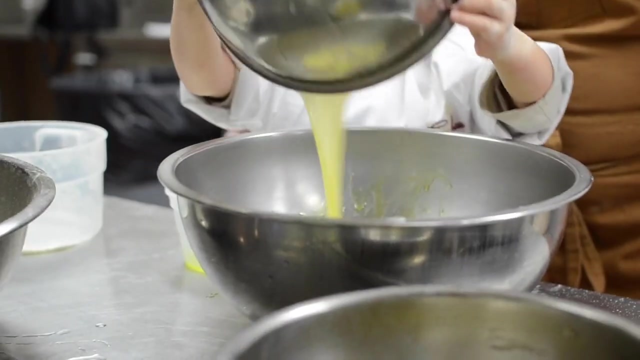 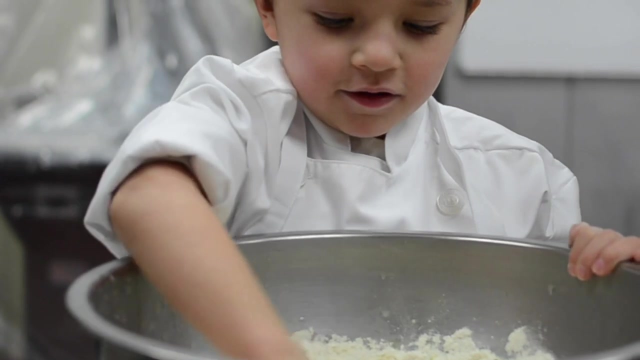 Wow, Five minutes is it? Yeah, Five, yeah, Yeah. Also, they're learning about different cultures, different ingredients, that they actually are going to take this for their recipe. It's part of their life. You know, when I was a kid, I used to cook with my grandma and my mom, and it's just fun. 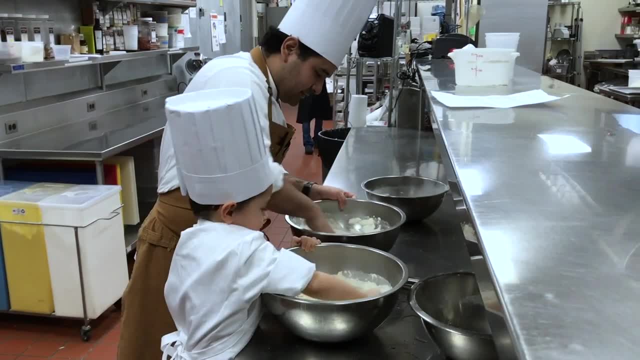 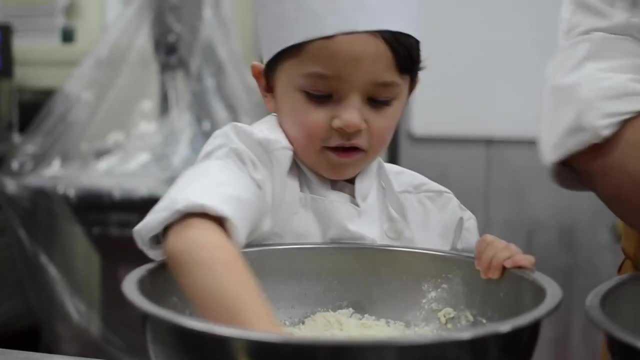 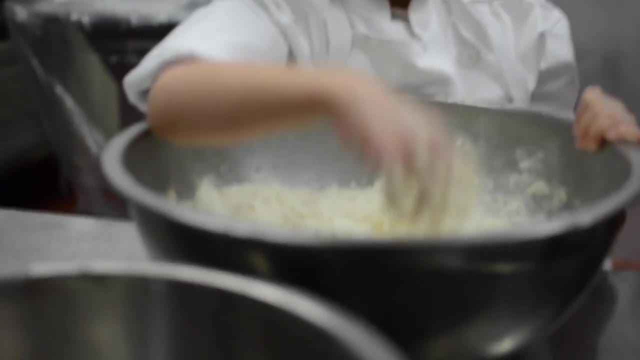 And my first experience in the kitchen was when I was five years old. My grandma- she's actually the one that taught me how to you know, cook. And then I get to experience with you know, different kinds of tomatoes, different kinds of- you know- vegetables that you know. 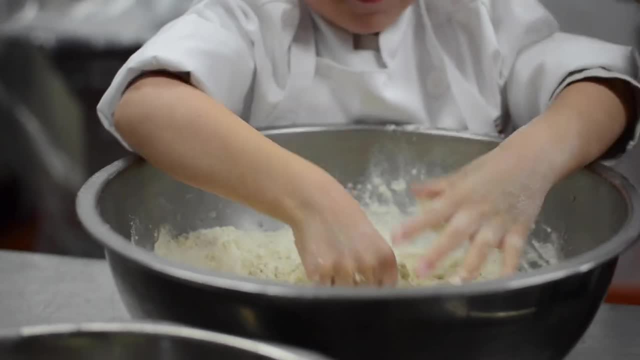 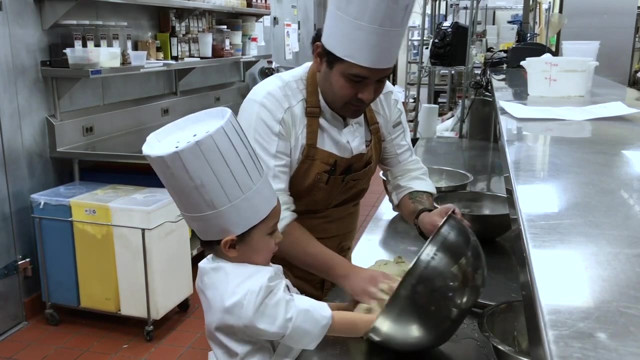 as a kid. sometimes you don't know, you don't want to eat because it looks. it looks, you know, weird in you know certain ways. But once you get to work with it and have your hands on it, it's when you realize you know as a kid you're like: oh yeah, it's fine. 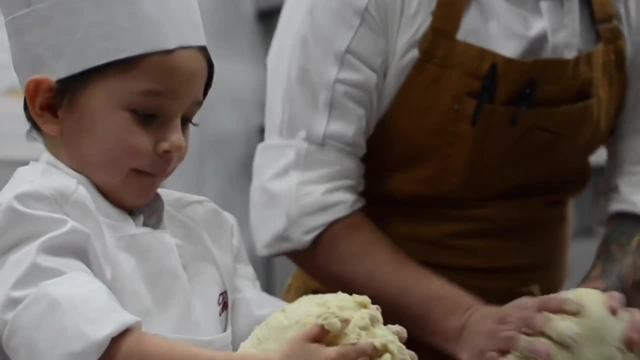 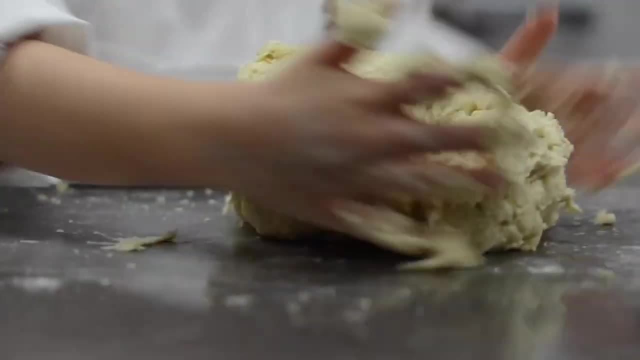 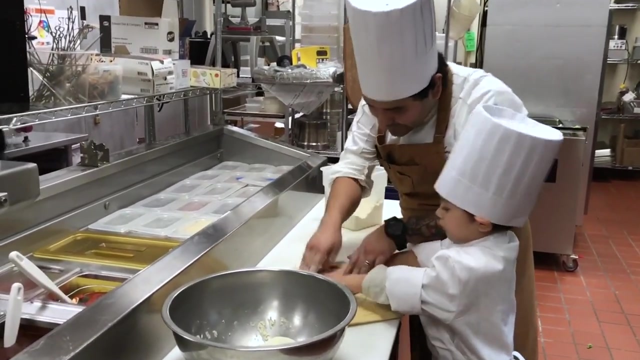 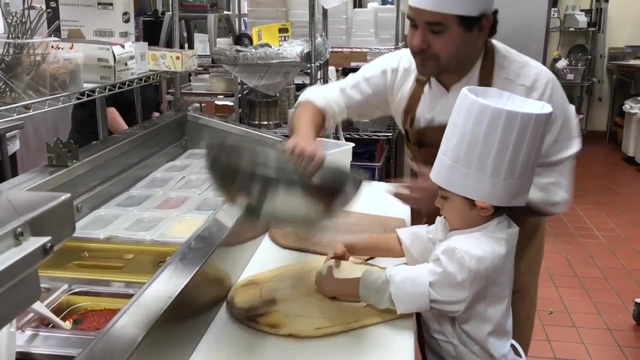 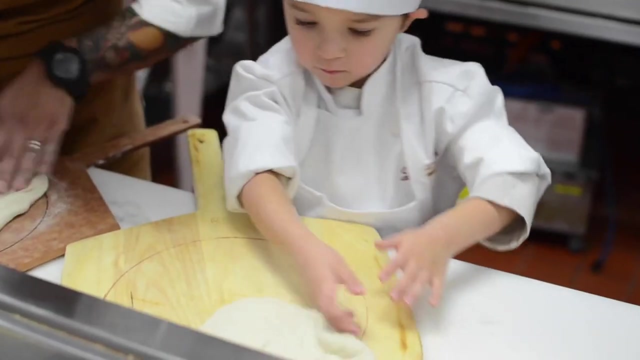 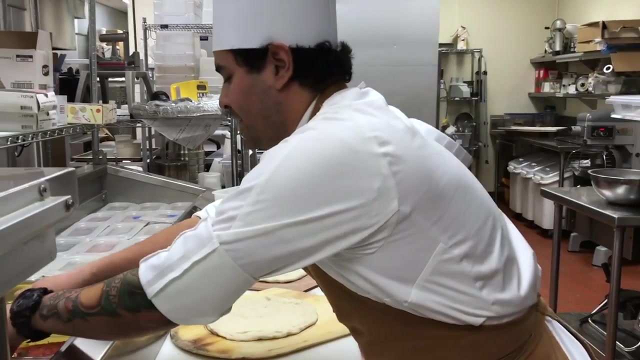 It's edible and it's good, you know, because I made it. I made it myself and I want to eat. Having a kid in the kitchen and you're at work, it's a different experience. It's something that you share with a kid. 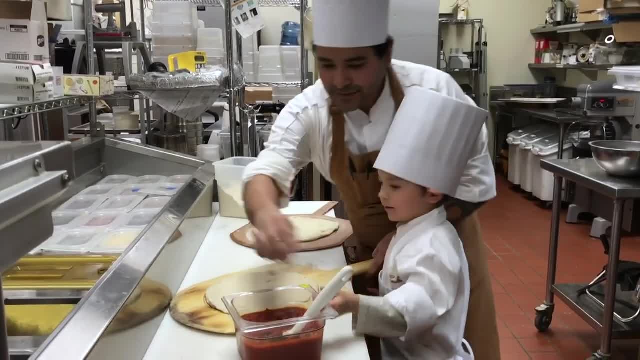 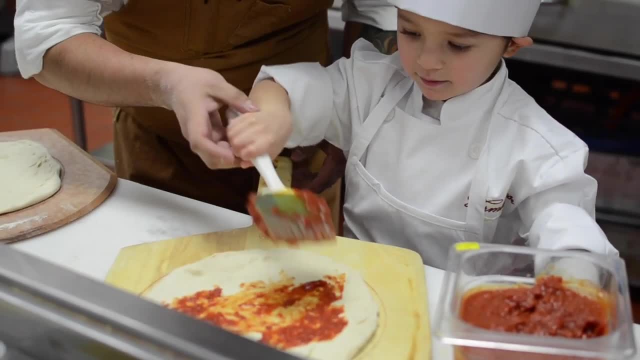 that it might impact their life. You know they might take it, you know, like I said, forever, because you're going to use those skills. you know who. hopefully, you know he's going to be cooking pizza at home when he grows up and show. show them, you know, to his siblings. 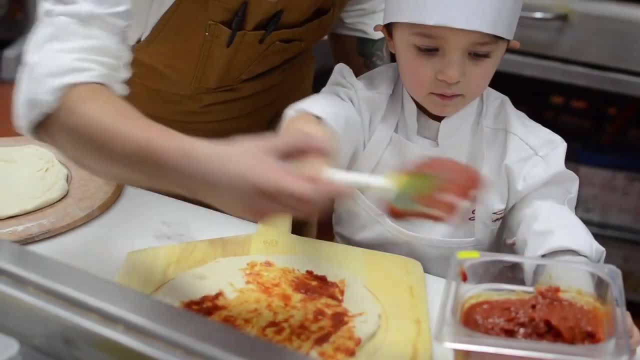 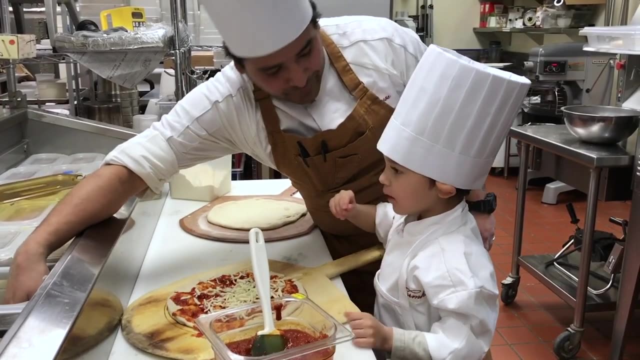 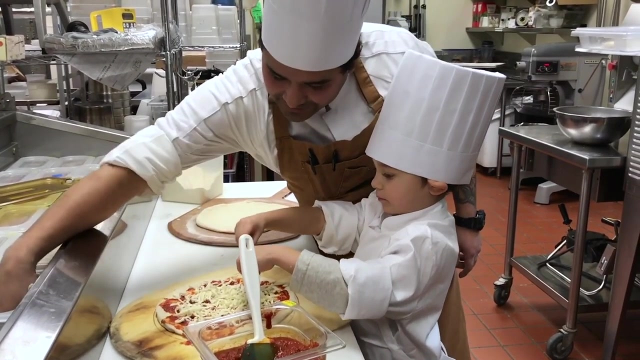 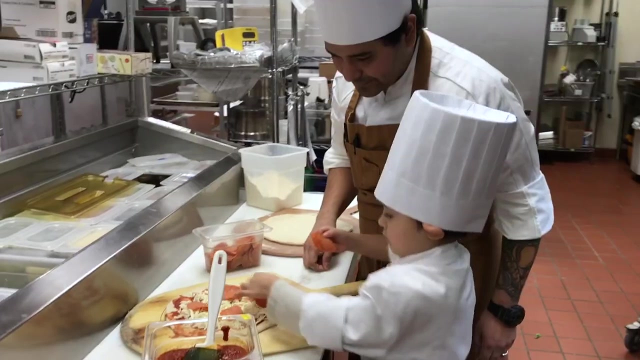 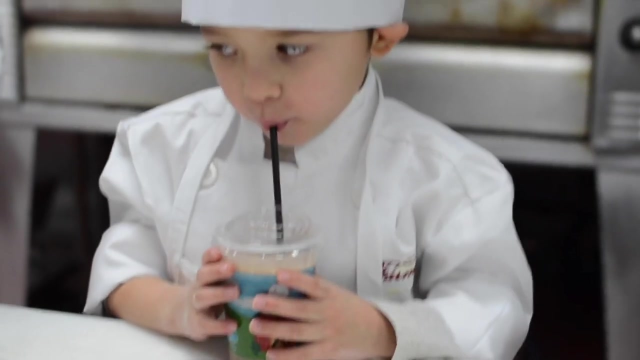 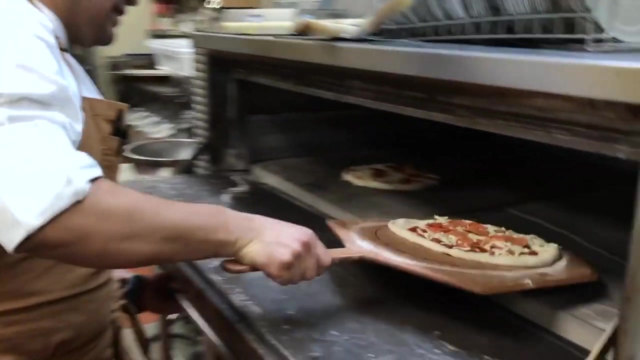 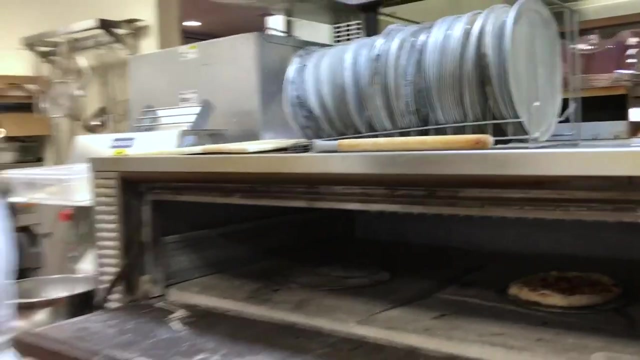 or you know, to his parents. Why not, You know, like it's something. it's something that I like to share. he did awesome, he is, he was amazing, he, he was listening, which is you know. 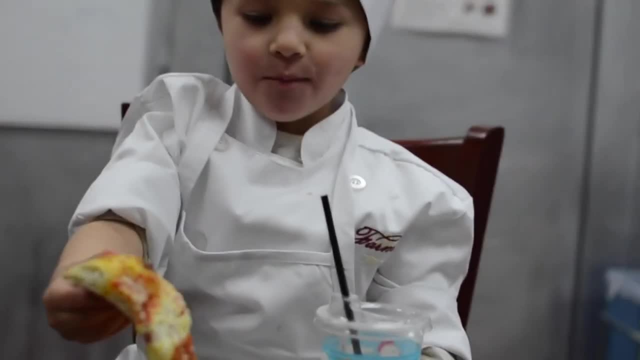 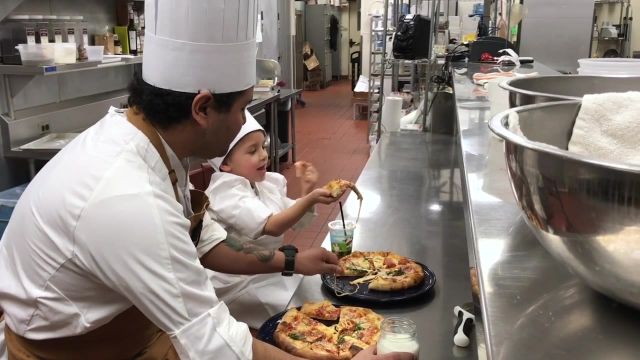 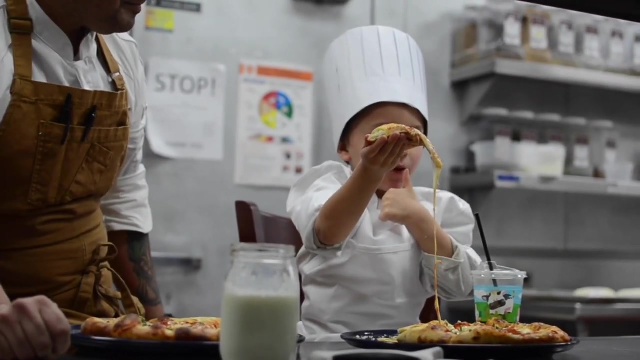 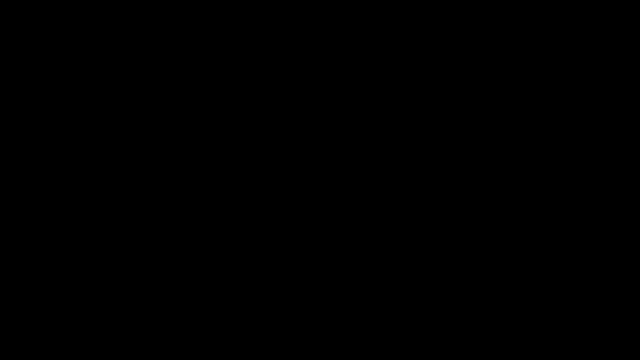 sometimes you know when, when, when you're dealing with kids, sometimes you don't know how they're gonna behave. you know, especially when you're. you know behind the cameras. but, um, he did, he did great, kid, he did great.